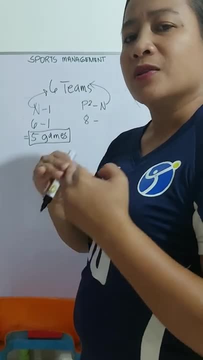 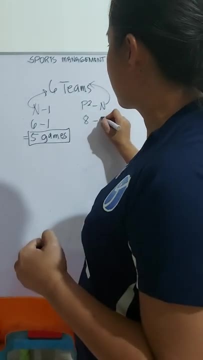 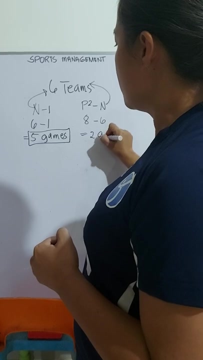 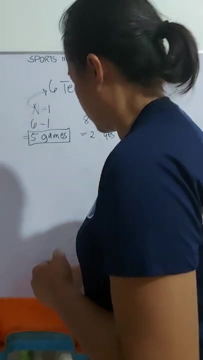 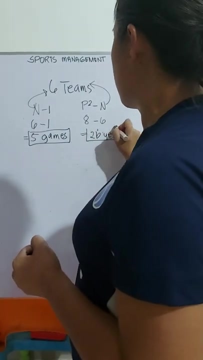 Four times two, it's eight, So on and so forth. So n is our power of two and n is six. So eight minus two, or eight minus six, So n is two by. Okay, there are two bys in six teams. 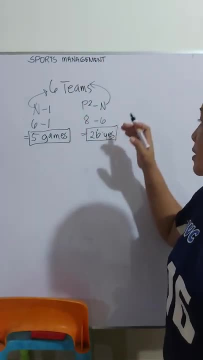 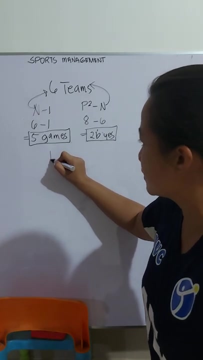 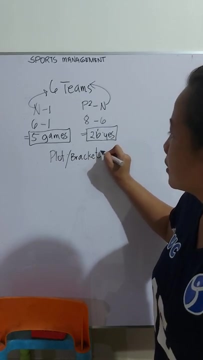 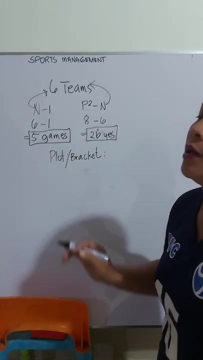 Now, after computing the number of games and also number of bys, let's try to plot our teams. Let's try to do this. So what we're gonna do, Let's try to take this number of teams, Let's put it into a pot. 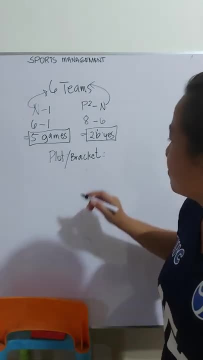 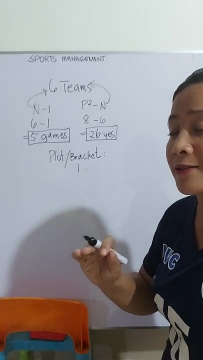 We're gonna put them in the pot And what we're gonna do is: you have to make sure they're not Wedge, That's right. So what we're gonna do is make the number of teams work In Q1.. 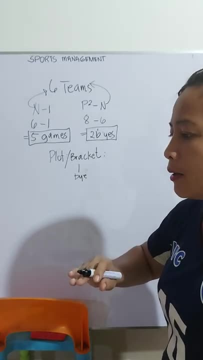 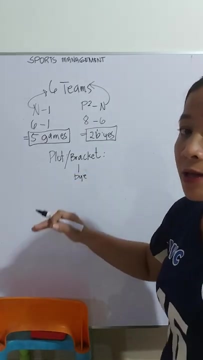 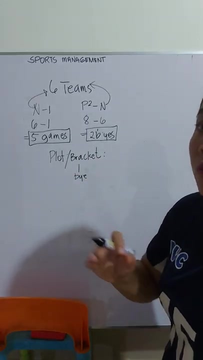 In Q2.. In Q3., In Q5.. So it works: buy under team one. so doesn't mean that team one is on top considered as the winner in the first round. no, it's not meaning to say team one is moved to the next round, advanced from the other teams. 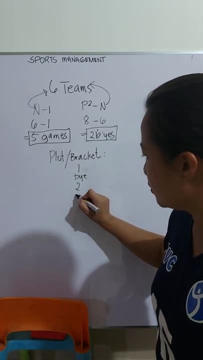 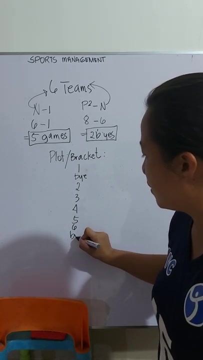 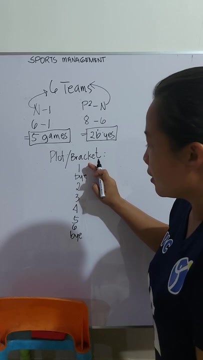 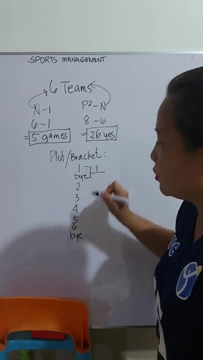 how about team two? let's say team two, three, four, five, six, bye. as you can see, we have two buys, and so our buys are team one and team six. and now let's close the bracket. this one is moved to the next round. by the way, this round is our first. 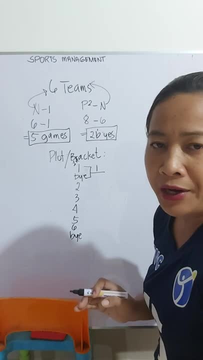 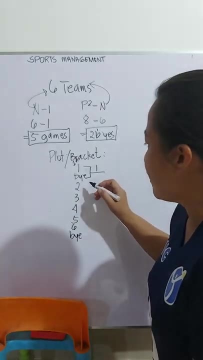 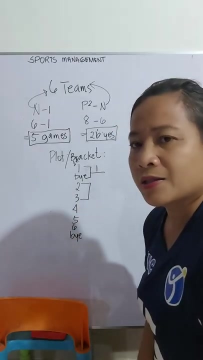 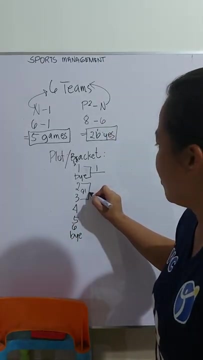 round, but no need to write first round there. it's just a an idea, so that we could easily identify it, that we have first round, second round, so on and so forth. so how about this? this is a game two versus three, so we have game one and so, after which, of course, there's a result which is winner one. 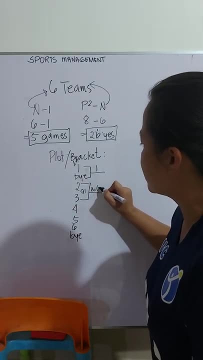 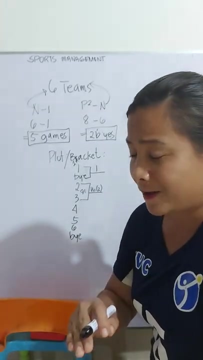 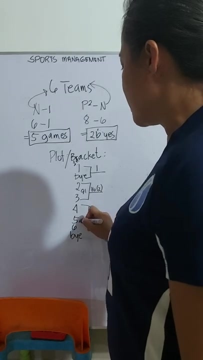 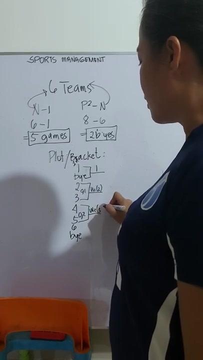 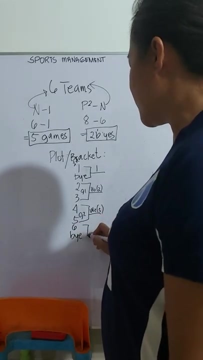 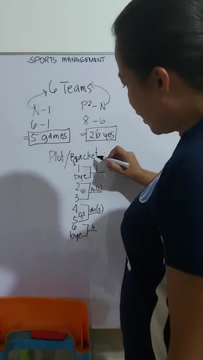 so, supposing our winner one is team two. so since this is single elimination, which is knockout system, automatically the loser is eliminated. how about this? this is game two. who is our winner two? supposing team five, meaning to say team four, is eliminated. now, how about this? just like team one moved to the next round. now let's proceed to the second round. 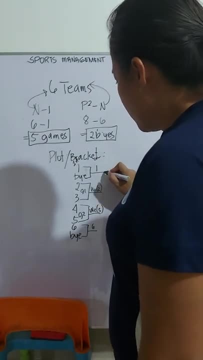 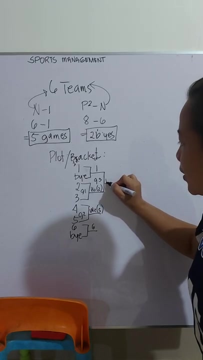 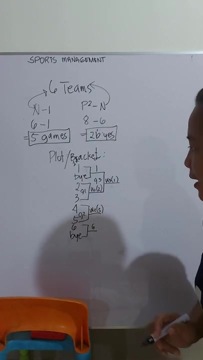 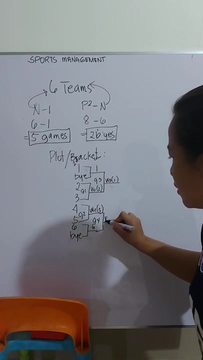 actually this is our second round. let's close the bracket then. this is our game three. let's say, winner three is our team one. so team two here is eliminated in game three. this one is game four. we have this. winner four, team six. okay, and now remember. 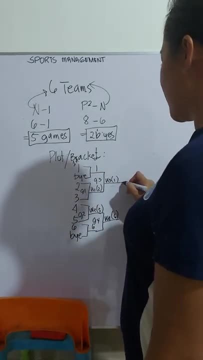 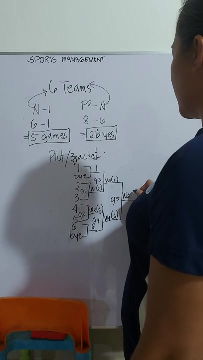 that we have five games all in all. so let's close the bracket. this is our game. five game, five, winner, five and let's say team one is the winner. implant our pickup system. this doing is we change this again. so team one is the winner wanting in this round. so 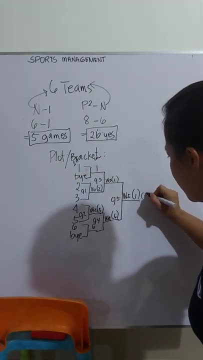 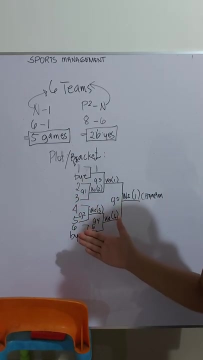 you wouldn't exercise you. so, with the regular checkbox, have minimum friends, the right hand, right hand, AND move the game from the left right hand. If you don't say that it's nola students champion. so that's how you bracket or plot the teams based on their category. so i'm using 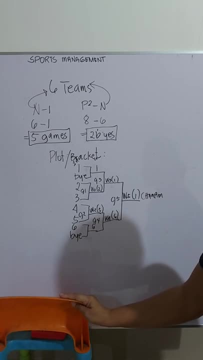 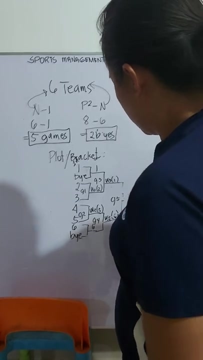 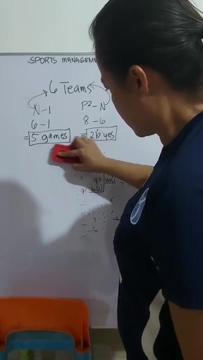 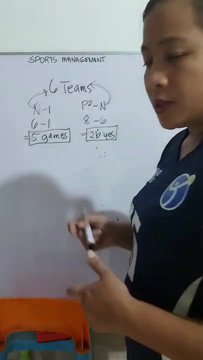 numbers, because it's easy for us to do it in order, whereas names probably you can place. you can place number in the names, but this would be easy for us to use the numbers. so i'll give you another example, aside this one. so the same six teams.